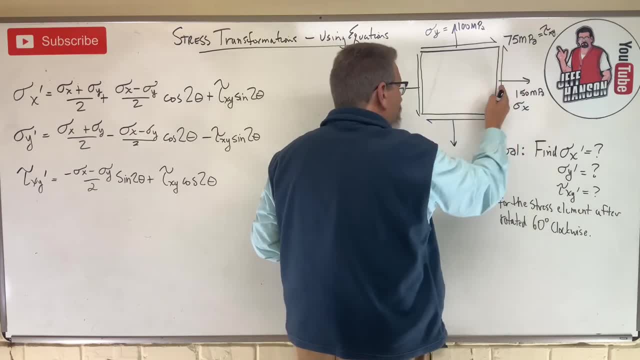 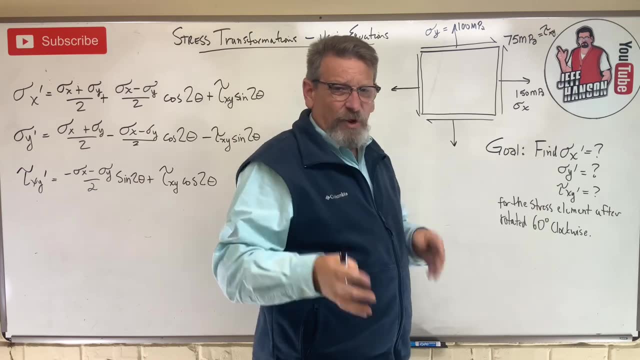 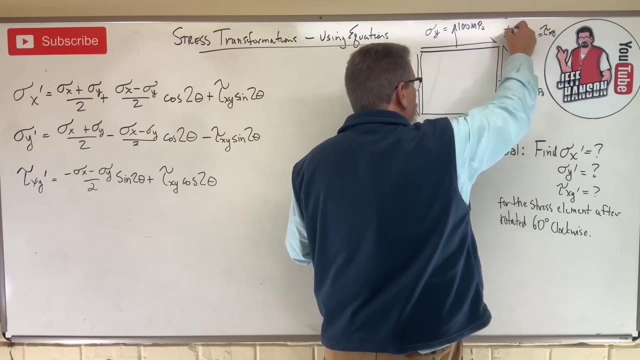 This guy right here rotates me. Think about this guy right here, He would rotate that element. what Clockwise? Just think about moments, right? A clockwise moment is what Positive, right? So anytime this, the sheer stress, goes to this corner, it's positive If it goes to this corner. 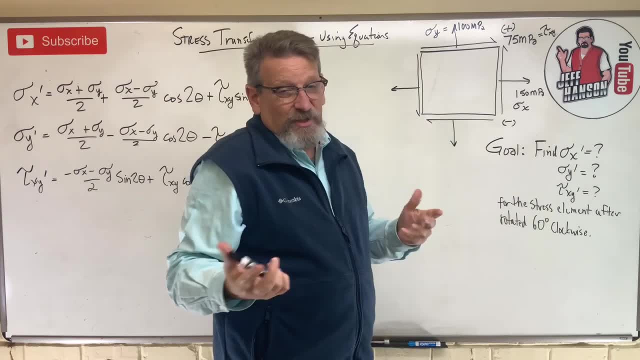 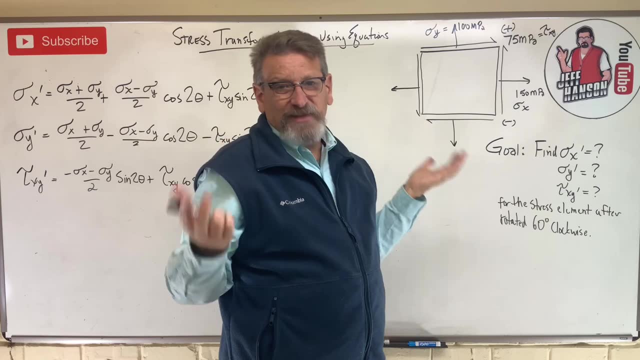 down here, that x face would be negative. So this guy right here, he would rotate that element negative. But you can just think about it like this way: Which way does he make me rotate? He rotates me counterclockwise. That's positive, Clockwise is negative, right Okay? 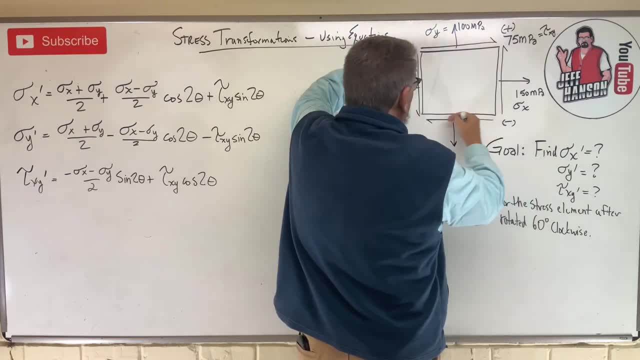 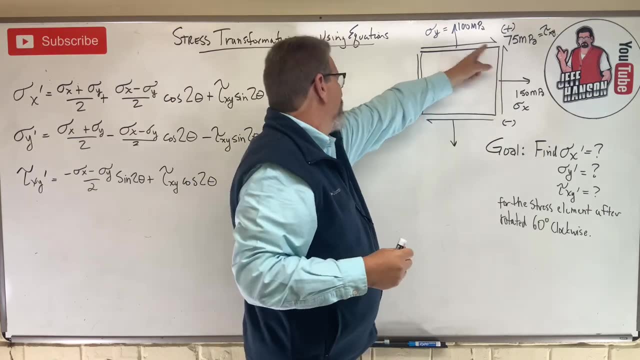 Well, how come these guys go together at this corner and together at that corner If the sheer stress didn't go in opposite directions? if it went, if this one went up and that one went this way, then that little element would be spinning right Is my little stress. 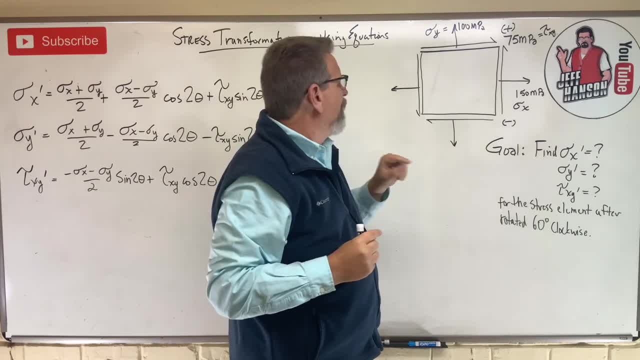 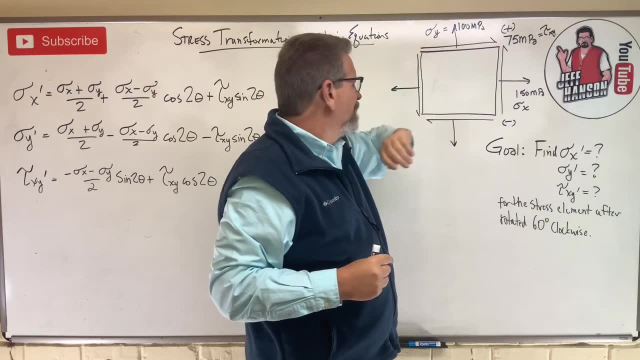 element, a little piece of material. Is it spinning? No, So if I have something that rotates me counterclockwise, I got to immediately have something that rotates me clockwise. And same thing: If I've got a force up, then I have to have a force down to cancel it, right? 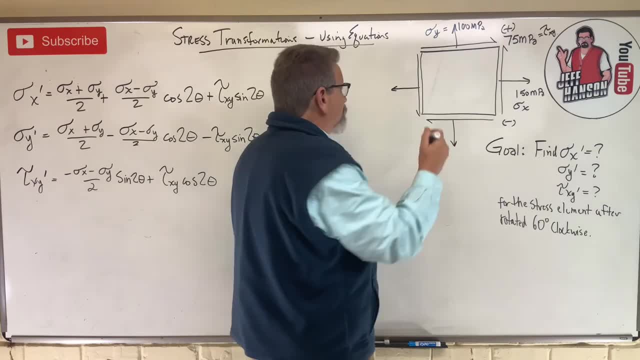 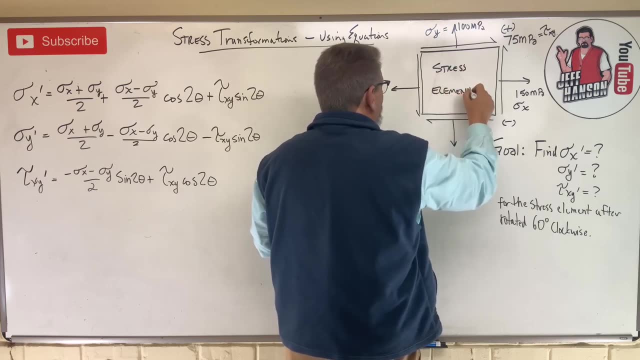 So that's what your stress element is going to look like. This is called a stress element. Okay, And in the last chapter, when we're talking about combined loads, what do we do? We took a real stress element and we're going to take a little stress element. And if we're going to focus on that then we're going to do that. RC found on that�s it We're going to take aς's cancelling and feelings on 가는 accounts and that's what we'll do And that's what we're going to focus on. So three pieces for the 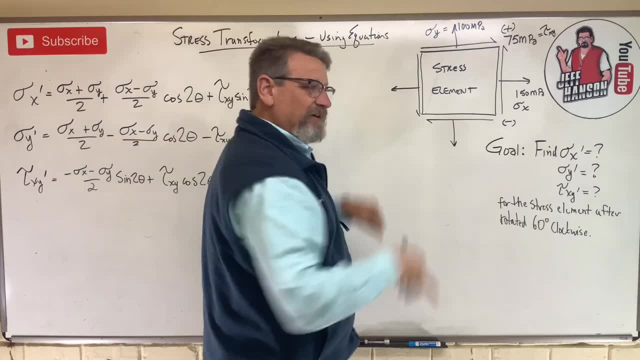 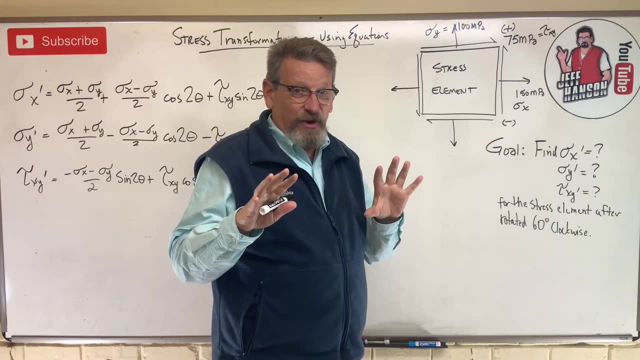 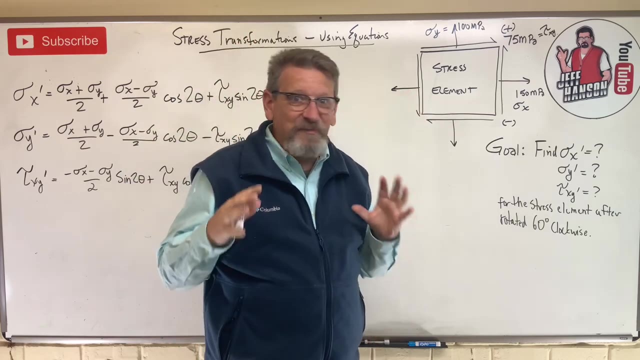 do we do? We took a really complex problem and we derived a stress element from that complex problem. Now, here is the first time that I'm going to tell you this. okay, Are you ready for this? Stress is directional. What does that mean? It means this: If I take this stress element, 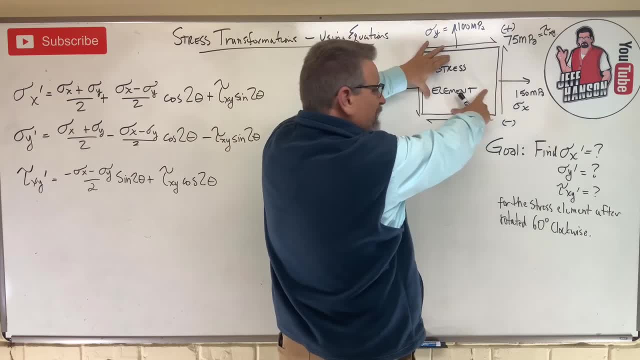 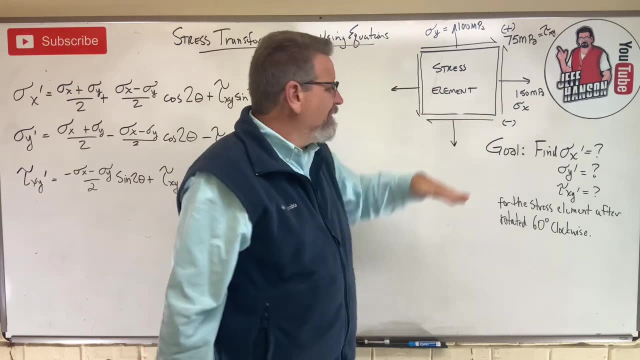 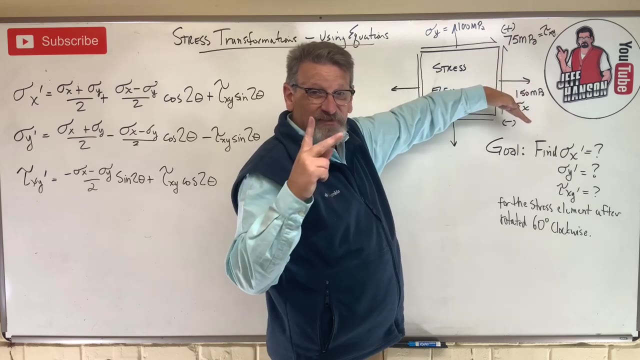 and I start to rotate it. let's say, I just rotate it 30 degrees clockwise, like that it's not going to have the same stress on it that it did here, right, Think about that: 150 megapascals, As it starts getting at an angle. then it starts having two components. It has an. 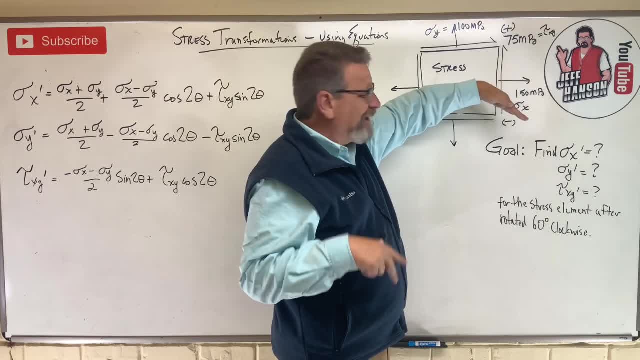 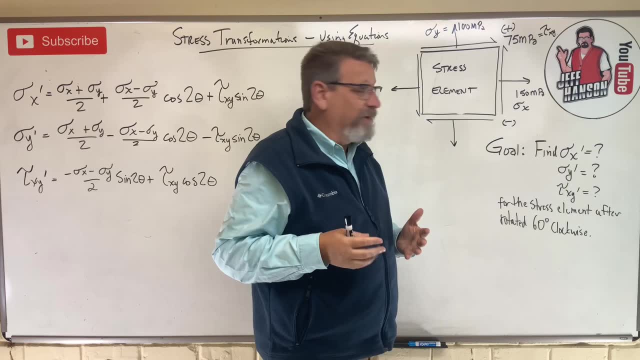 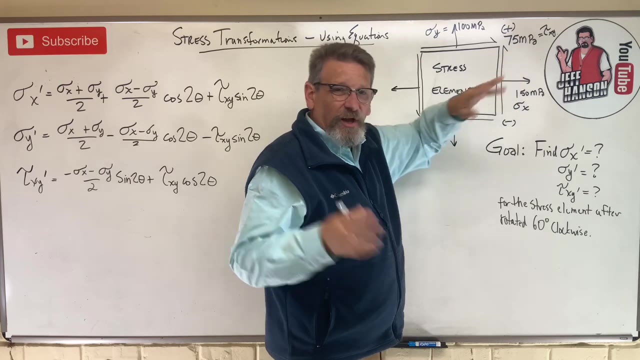 x and a y component. Instead of it being all of the x, now it's got an x and a y. Well, the y part of it turns into shear stress. right, That one component, instead of just being all normal stress, now part of it, turns into shear stress. So this goes down, that goes up. 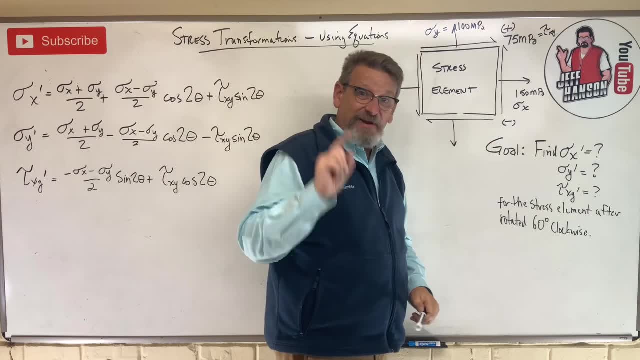 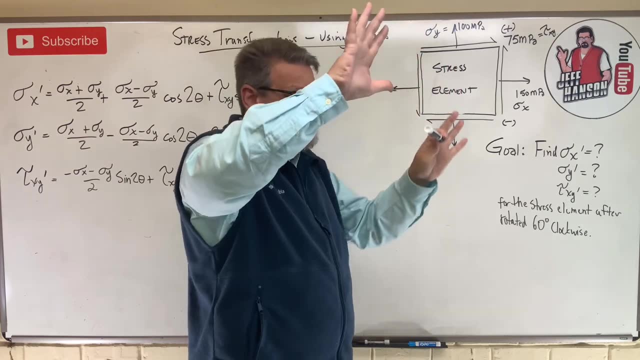 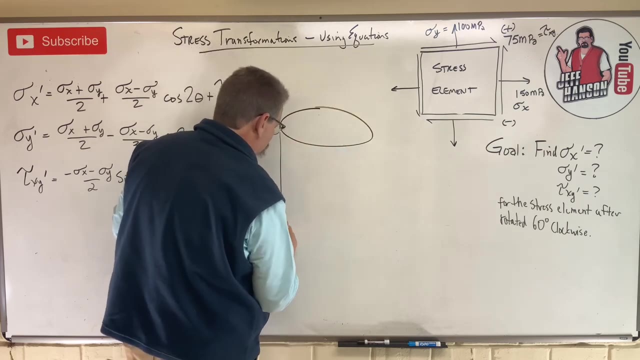 everything starts to change. okay, Stress is directional, So sometimes we want to know what is stress at this angle, What is it at that angle, What is it at this angle, Okay? so think about like this: okay, I've got a big like holding tank, okay, And they made me go out. 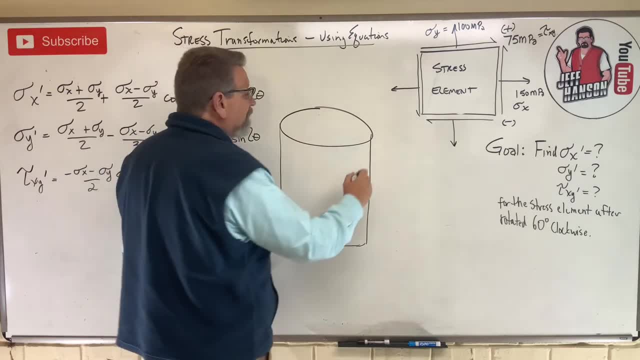 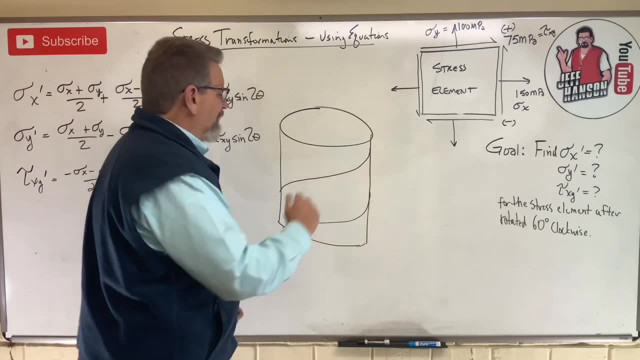 and weld this thing together, but all I had was a strip of steel, And so what I did is I took my strips And I welded them together like this, right Into a big spiral. okay, Now, when I look at this, 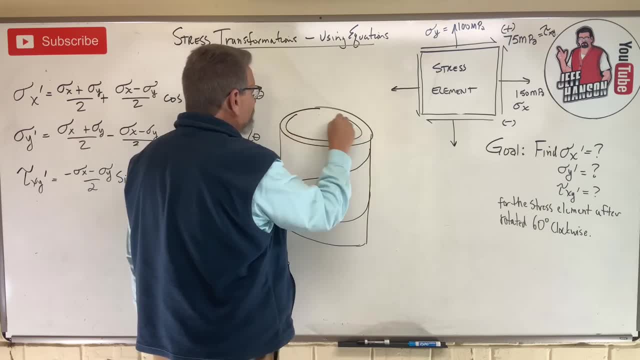 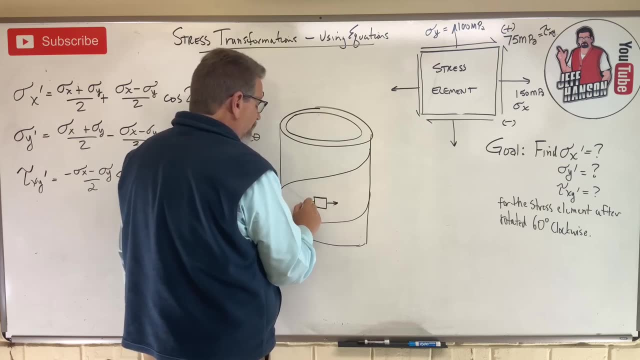 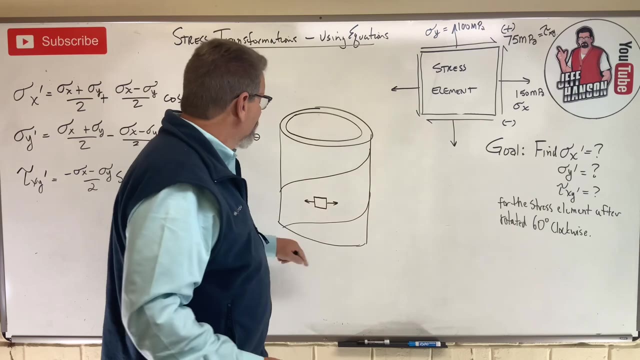 cylinder here, if you will, this big holding tank. if I look at a little piece of material right here, you know it may have a little bit of this on it. What is that called? Oh, there it is. It's hoop stress, right, Hoop stress. So that may be putting me in tension. this. 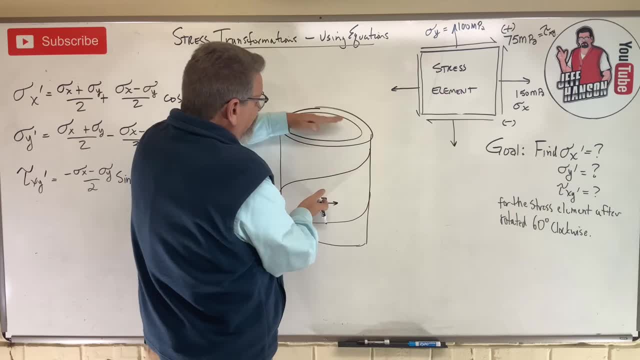 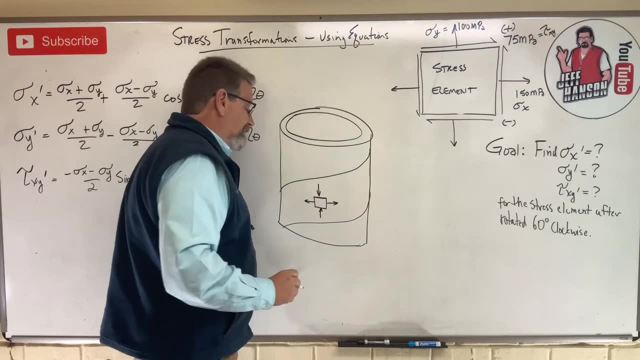 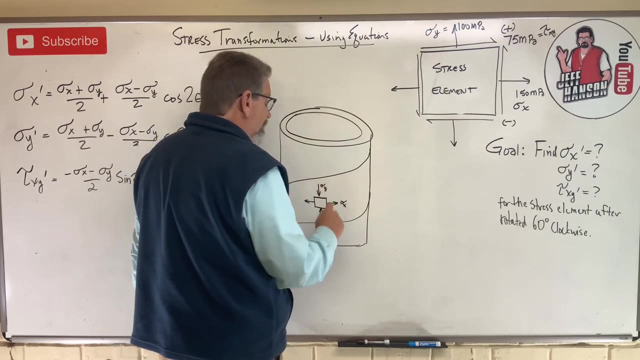 way. What about this? If I'm a piece of material, I can feel the weight of all this steel above me, So I might feel a compression in this direction. okay, Now, if I had, this would be sigma X and this would be sigma Y. Maybe I don't have any kind of torsion or anything like that, So I 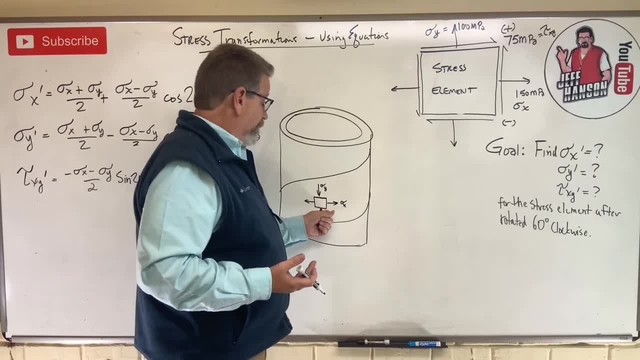 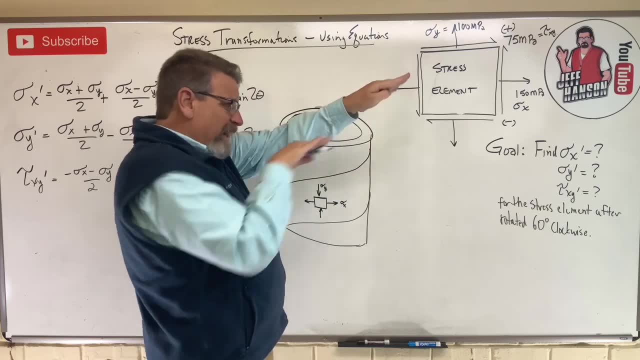 wouldn't have any shear stress whatsoever. But what about? the welder comes back and he wants to know like how much shear stress is there. And he wants to know like how much shear stress is there that's going to tear my welding apart on this joint right here. So maybe I want to know. 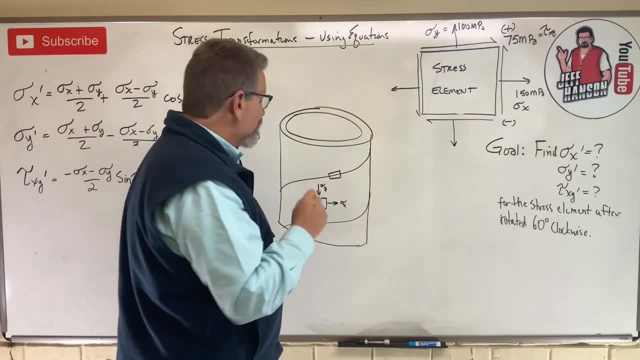 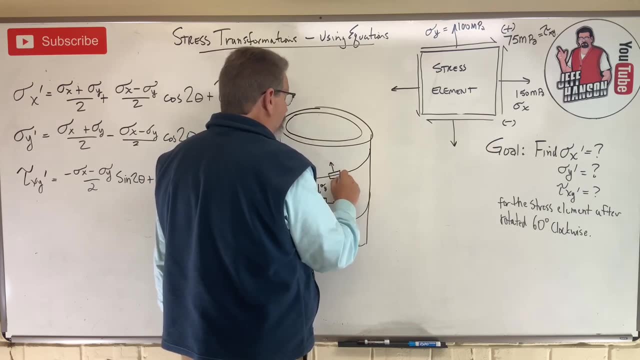 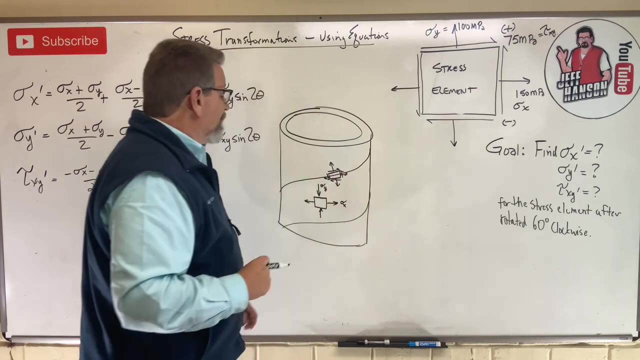 what is a stress element that's aligned with the joint at some angle, right? What's going on there? Well, here I might have this, I might have this, and now I'm going to have a little shear stress around this thing also, right. So what if I wanted to know that? Can I take this guy? 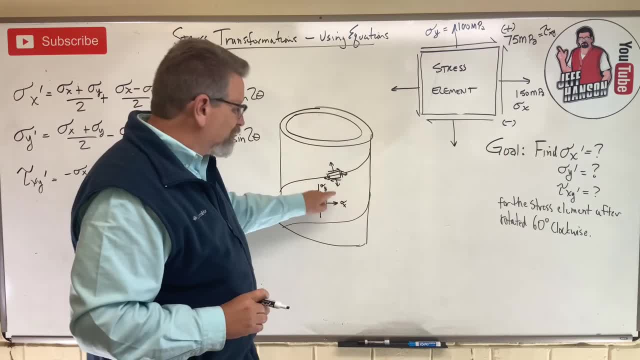 a stress element and I'm going to have a shear stress around this thing also. right, Can I take this guy a stress element and I'm going to have a shear stress around this thing also. that I know that I can calculate. I can calculate hoop stress, I can calculate weight of a material. 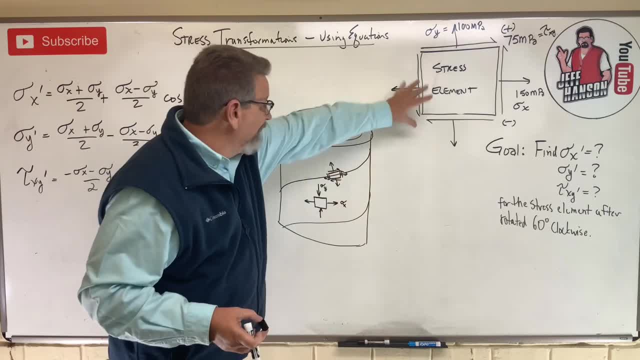 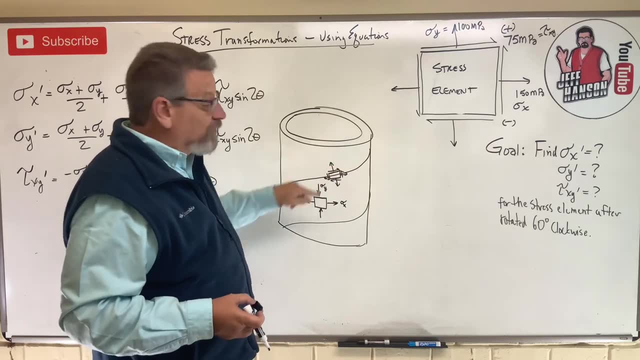 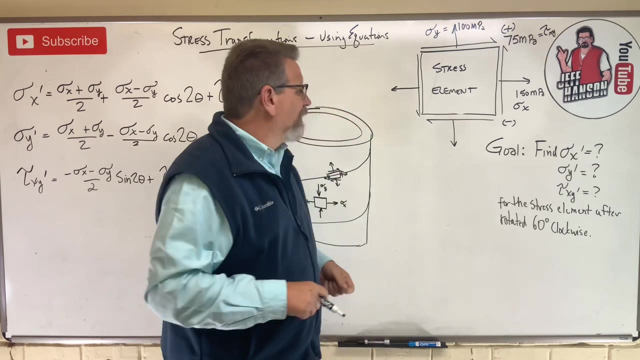 above me. Can I take that guy which would be like that and go whoop and spin it to that and be able to tell what these numbers are at a new angle? The answer is yes. The answer is right over there. okay, We'll talk about that in just a second. So let's look at this problem that we're 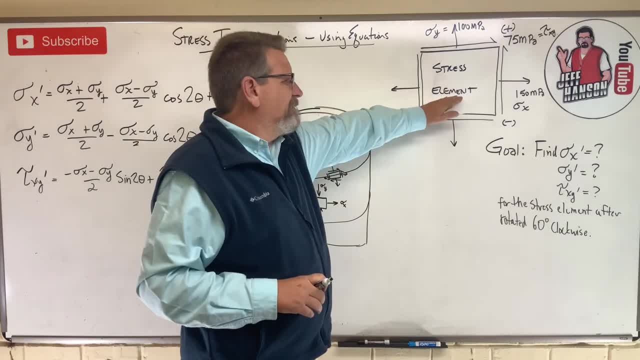 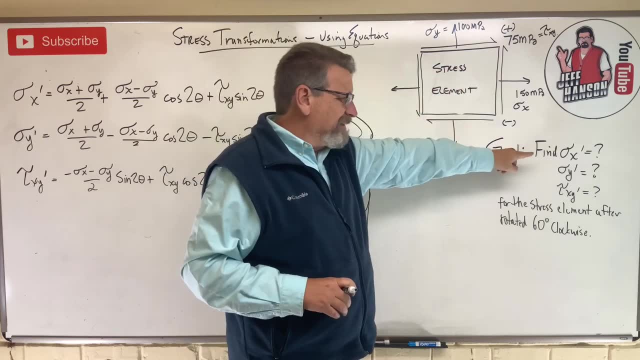 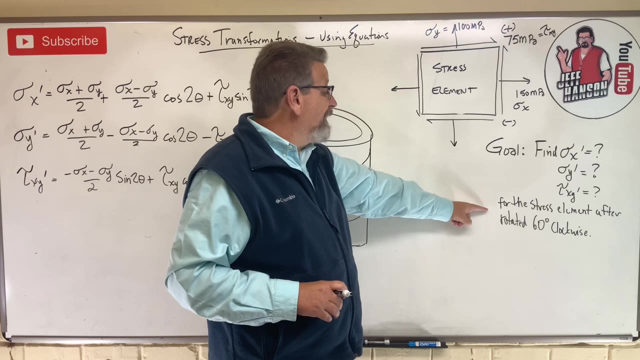 talking about here. They gave us a stress element. okay, So we have a sigma x, a sigma y and a tau xy. okay, Look what they say: Find sigma x prime, sigma y prime, tau xy prime for the stress element after it's rotated 60 degrees clockwise. okay, 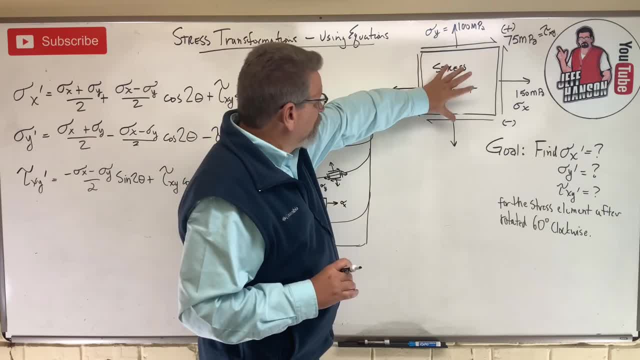 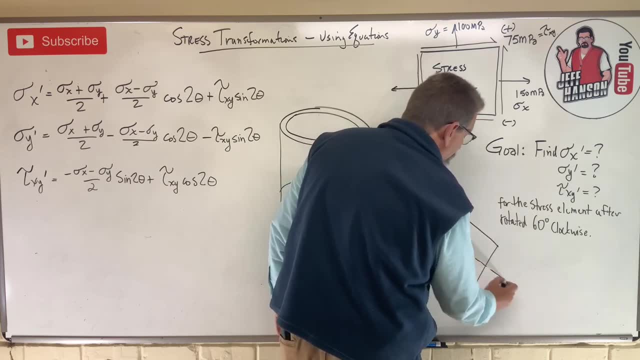 So we're going to take that element and we're going to go like this, and so now it's going to be like this: okay, So this from here. right, we rotate it this way: 60 degrees, and so now I have a new x and a y. 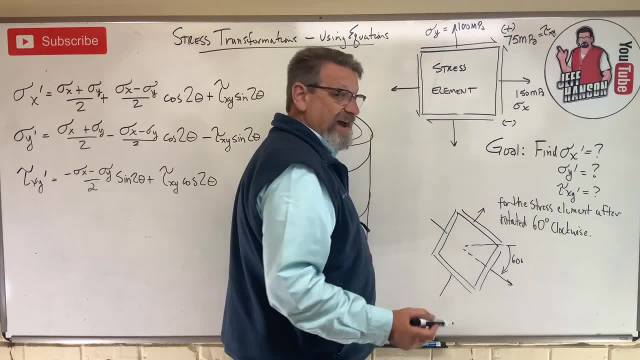 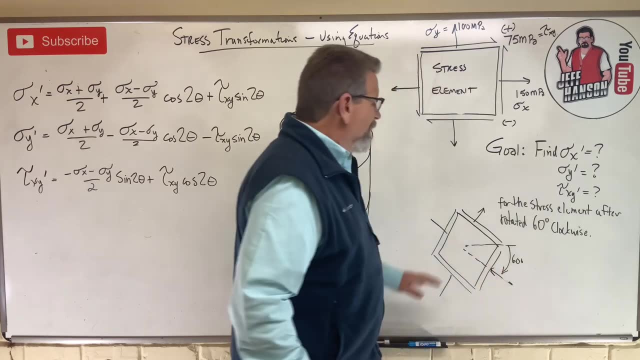 and I have a new tau. Now here's the deal. I drew that like that. That may not be like that, That might be like this. okay, We're in one at one angle. this was a positive right, which means: 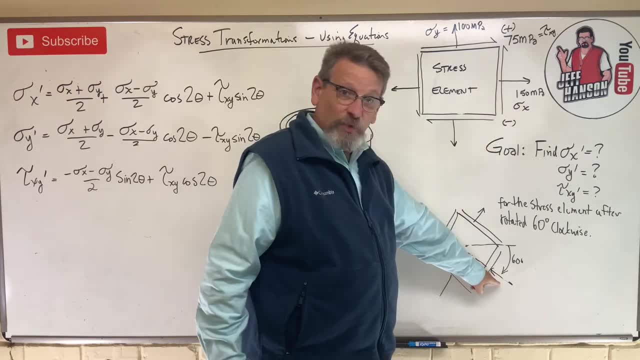 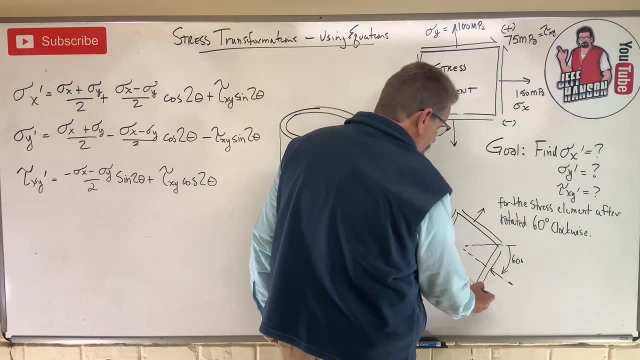 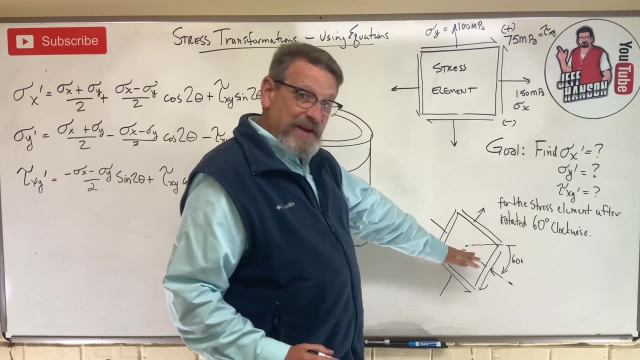 it was in tension. but as I transform it I might find that it switches over to compression. okay. And then same thing with tau. It's going up here, but over here it may go this way. I don't know, I'm going to have to solve for it Now when I transform it. it's not the same as 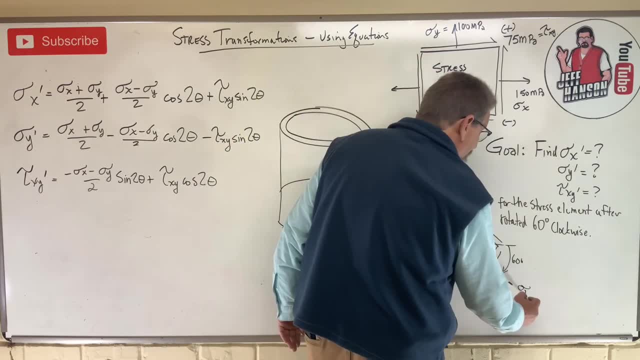 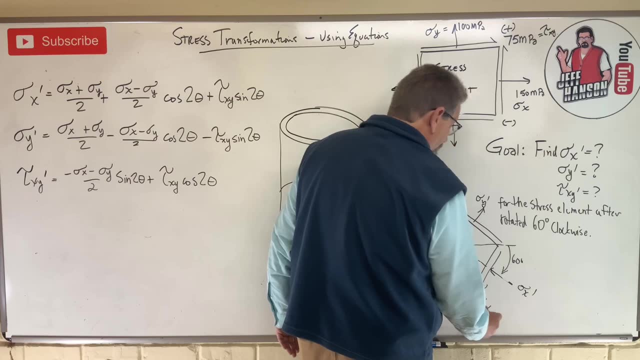 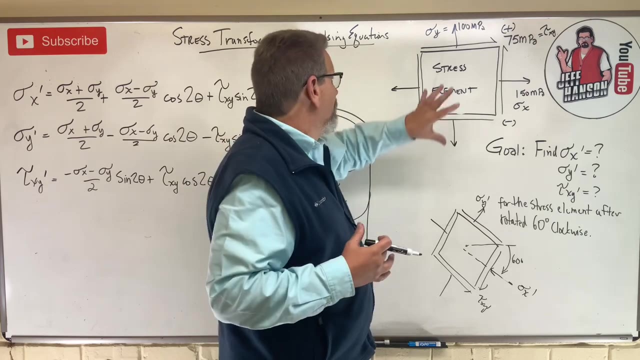 it used to be okay And that's what's called sigma x prime, sigma y prime and this guy right down here tau xy prime. So the prime is just an indication that it is a modified or changed element. When there's no prime, that's the given okay. The prime is the transformed numbers. 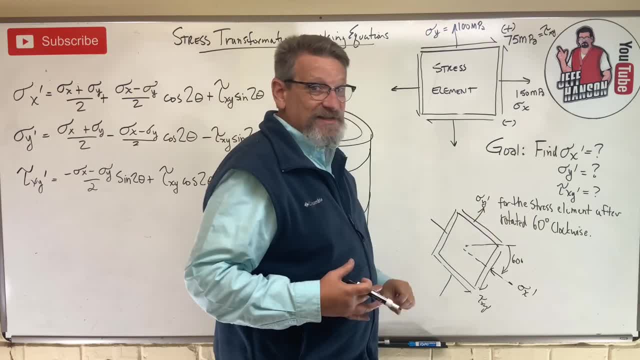 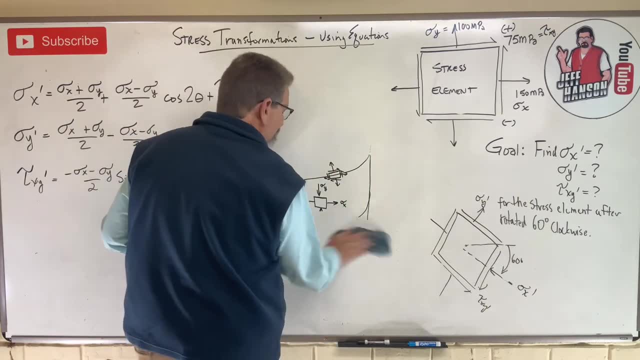 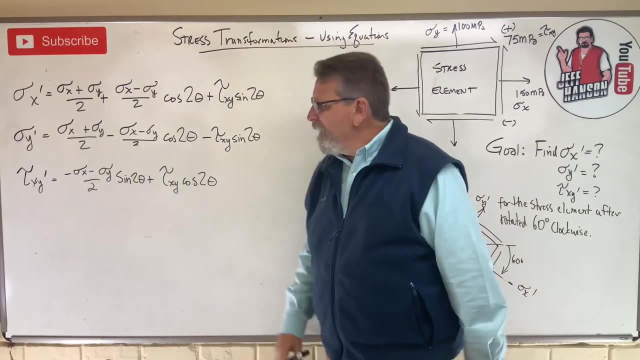 okay, So we're going to rotate it 60 degrees clockwise and get these new numbers. okay, So let's talk about our equations over here. Now I have to tell you this: okay, Confession time. this is not my favorite thing, okay, I hate it. You know why I can't remember those equations. 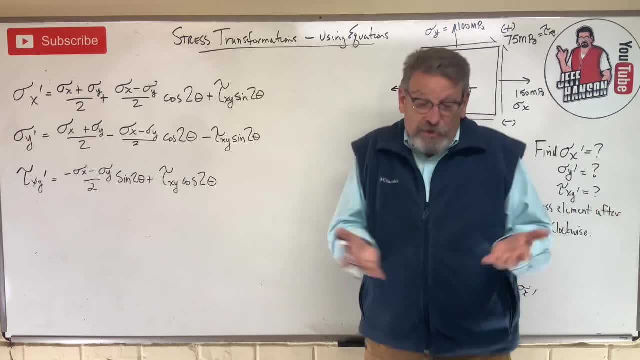 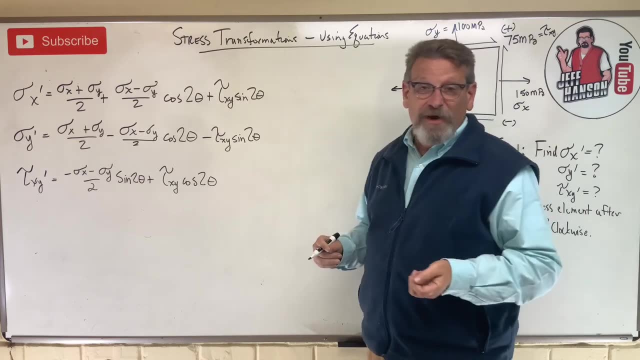 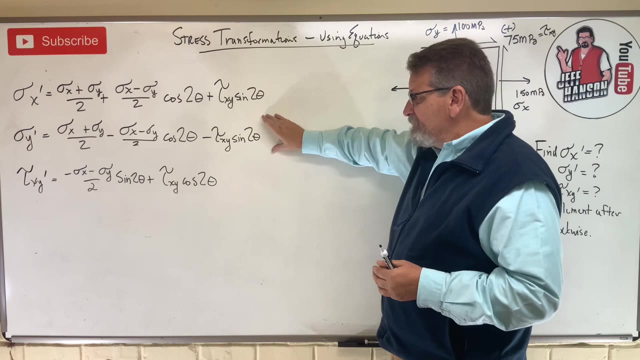 It's a Google world. You can look them up. They're on the internet. They're in your book, Hanson. are you going to derive them for us? No, I'm not okay. I'm sure there's a derivation somewhere, but there they are okay, And so these are pretty straightforward. This is sigma x prime. 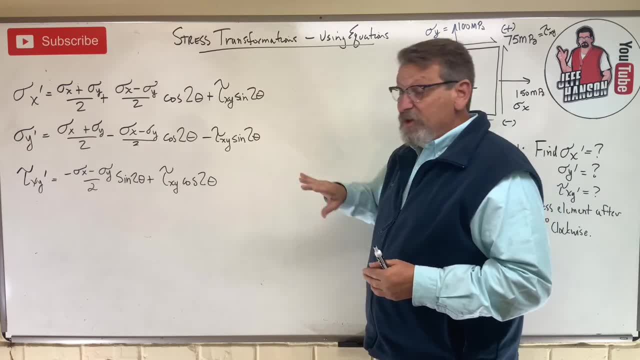 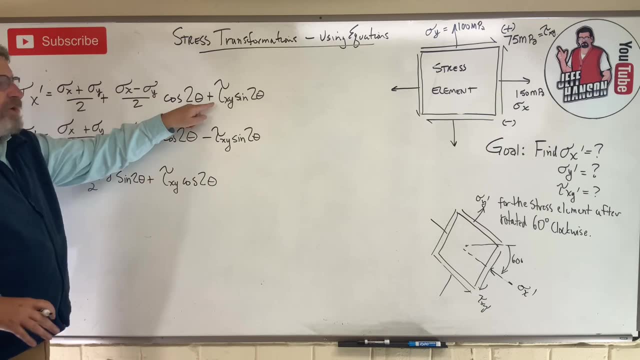 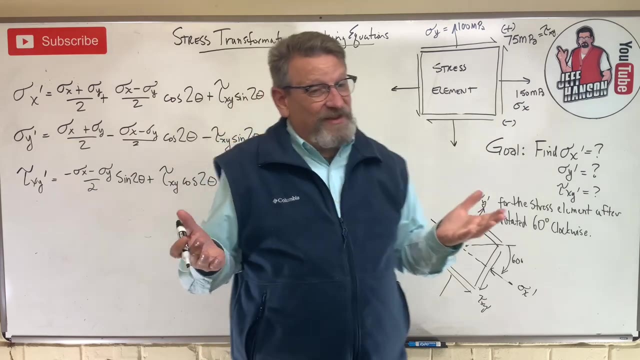 sigma y prime and tau xy prime. So that's what we're looking for. We're looking for this new number over here. But notice in the equation, these things here don't have primes on them. What does that mean? They come from here. Now the equation method. a lot of my students like the equation method. 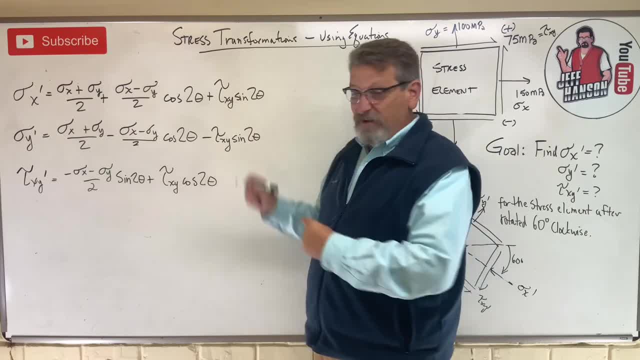 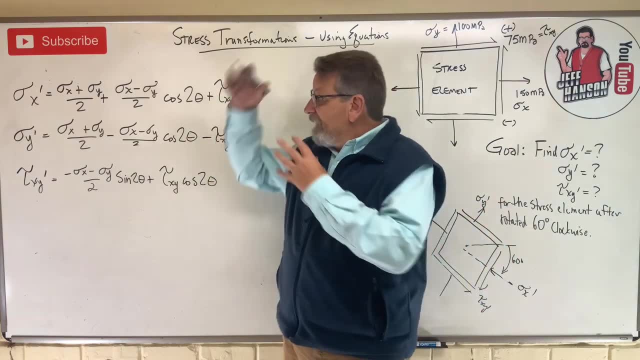 because it's as simple as taking those numbers, plugging them into there, put them in your calculator and get an answer. That's really all there is to it. okay, But the problem is that I can't remember these equations. Now, if your teacher, your professor, lets you have an equation, 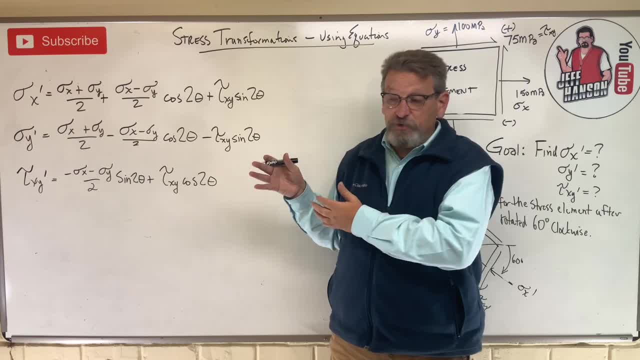 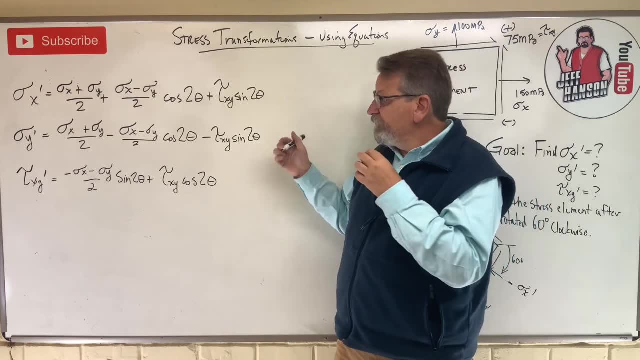 sheet. these equations generally are on those equation sheets. Their stress transformation equations are on the ones that are in the front of the book. I let my students have that, so a lot of students will just use this. I want to show you a method. It's about two videos away. 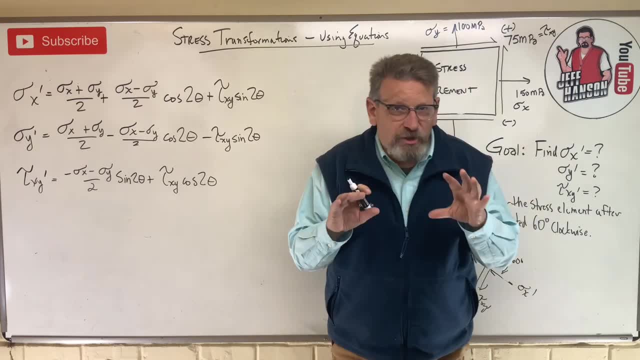 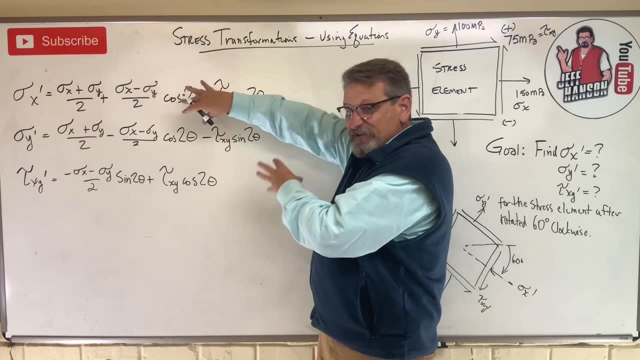 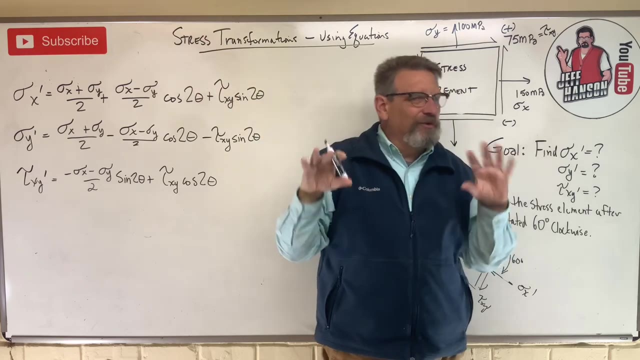 maybe three, but I think two called Moore's Circle, where we can do a graphical transformation and we can get all the exact same numbers that these equations give you without having to remember the equations, okay, So if this is kind of blowing your mind, stay tuned, We're going to. 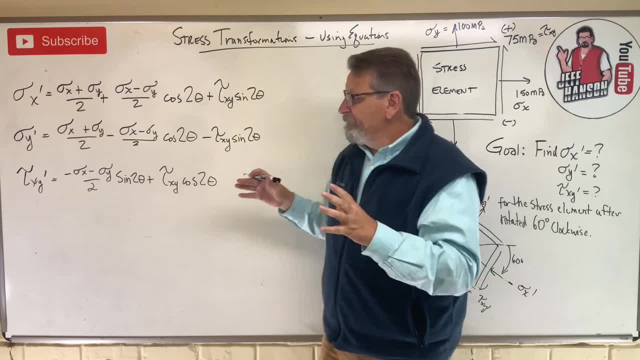 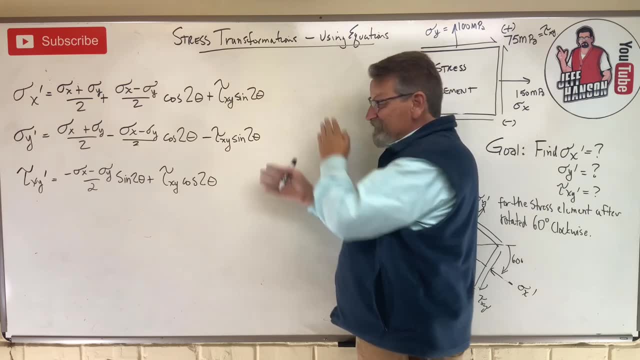 talk about another method where you don't have to do this. okay, I think this, my personal opinion is, this- is the Johnny Weak Sauce method. If you're a Johnny Weak Sauce student, you will just stick with the equations, but Johnny Genius student, he's going to do Moore's Circle. That's me, I like. 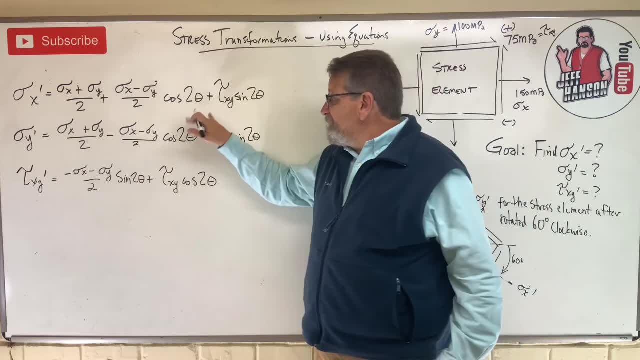 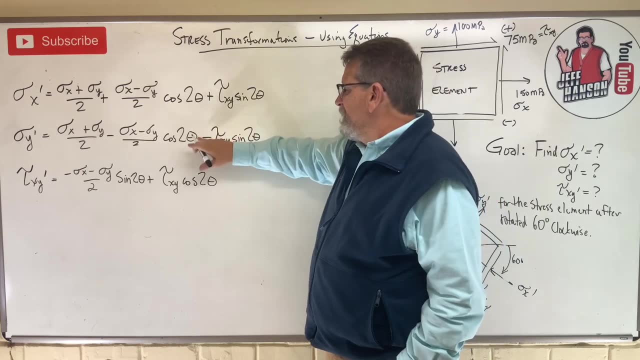 those. I don't like this because I can't remember them. So what happens if I put: you know what's the difference between x and y? Add 90 degrees to it, right? So if I put theta 90 minus theta here? 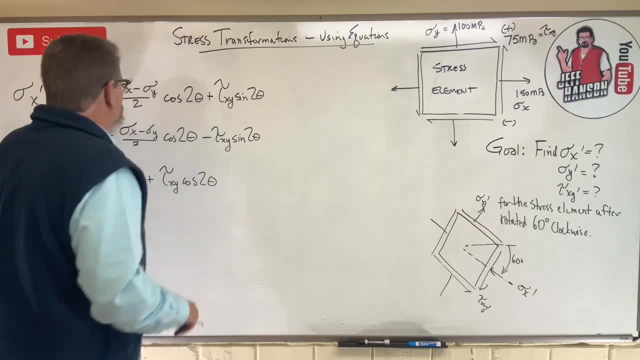 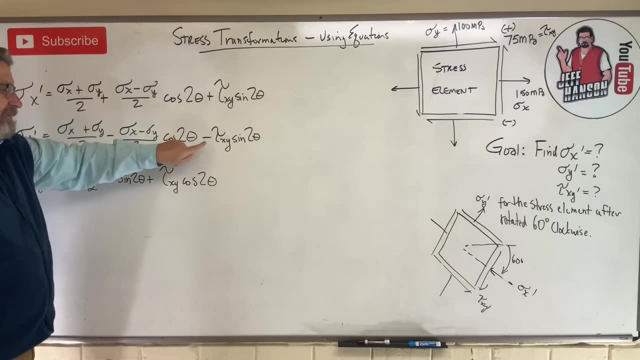 right, this just changes the signs. So the only different difference between the x prime and the y prime is: this is positive, that's negative. This is positive, that's negative. That's the only difference in those two. okay, And then the tau- xy equation. notice that these are signs, Signs. 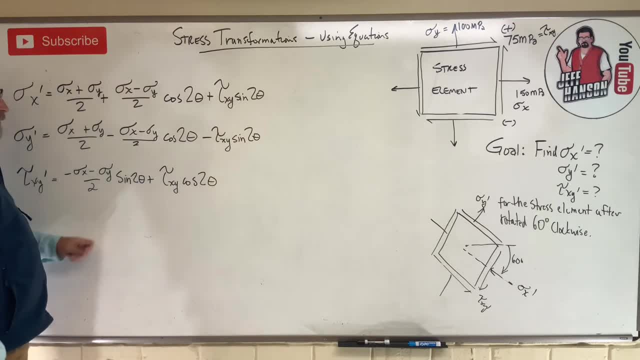 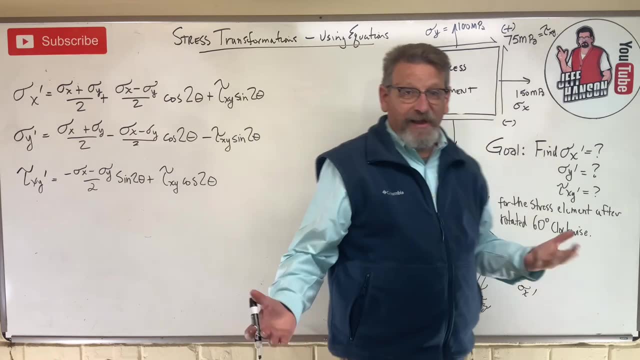 this guy is a cosine, okay, So don't mess that up. This one's different than these two here. If you have to memorize them, I hope you don't have to memorize them because I certainly cannot remember them, okay. So I don't know if you've ever done that. I don't know if you've ever done that. 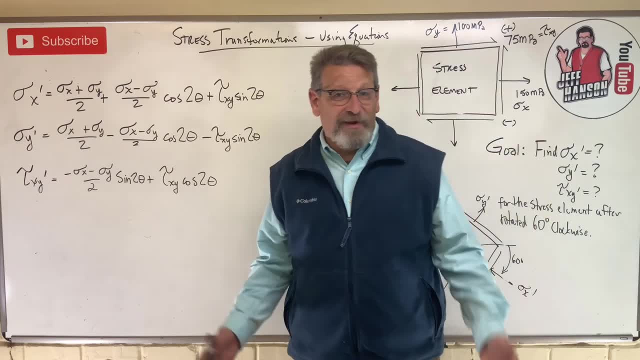 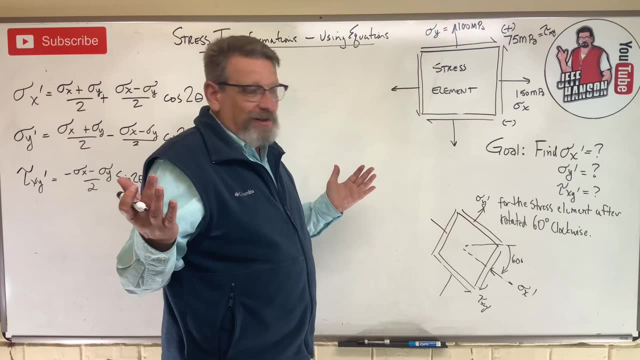 I don't know what else to do other than just let's just solve the problem that they wanted here. okay, So they want to know what is sigma x prime, y prime, tau xy prime. Let's just plug and chug. 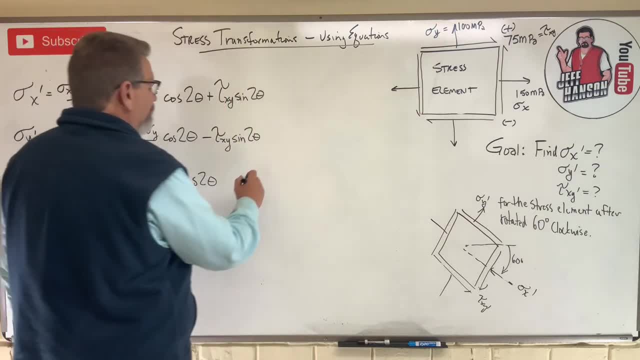 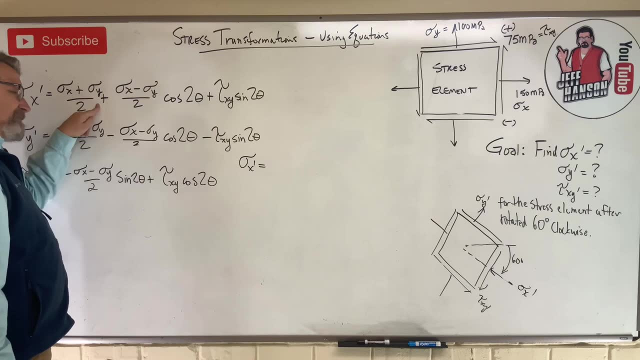 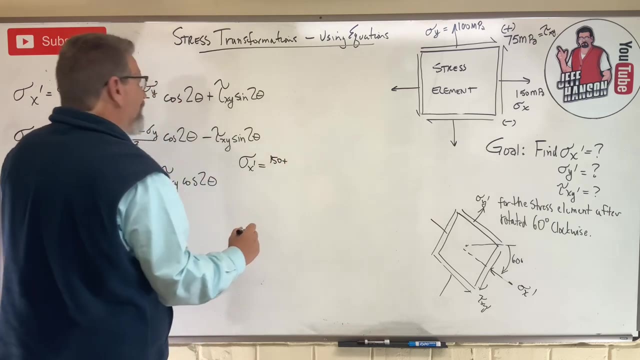 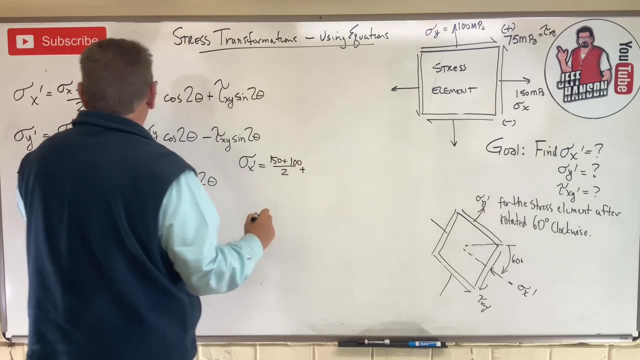 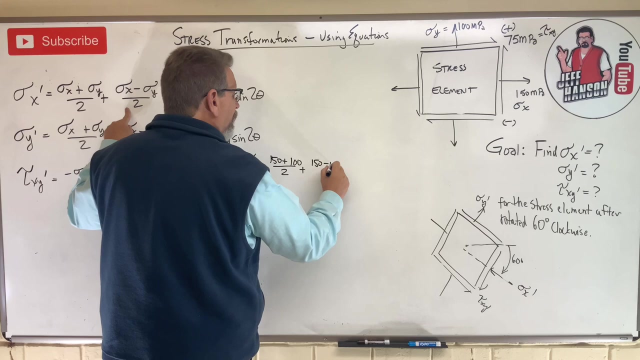 Let's get it done okay. So the first equation: sigma x prime is equal to, okay, sigma x plus sigma y. Well, sigma x, bam 150.. Sigma y, what? 100 divided by 2, plus right, sigma x minus sigma y. So 150 minus 100 divided by 2 times the. 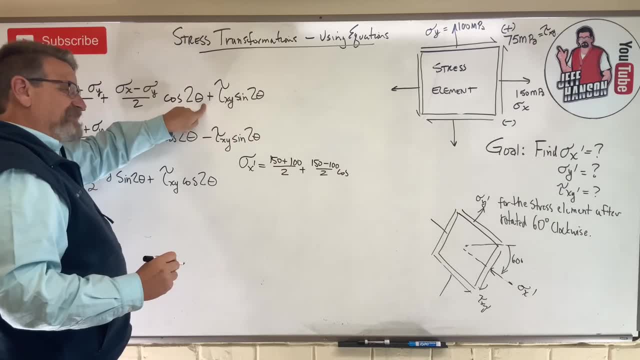 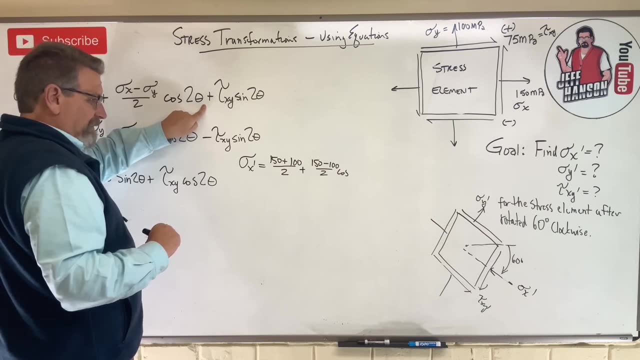 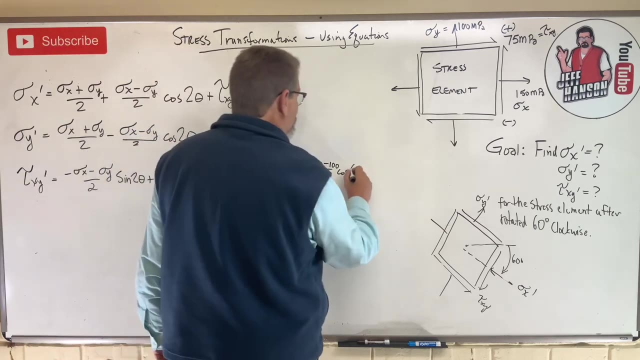 cosine of what? 2 times theta. Well, it said: rotate it 60 degrees, clockwise, okay. So what is that going to be? Clockwise is going to be what Negative, isn't it? So it's cosine of negative 60 degrees, right? Remember that, okay. 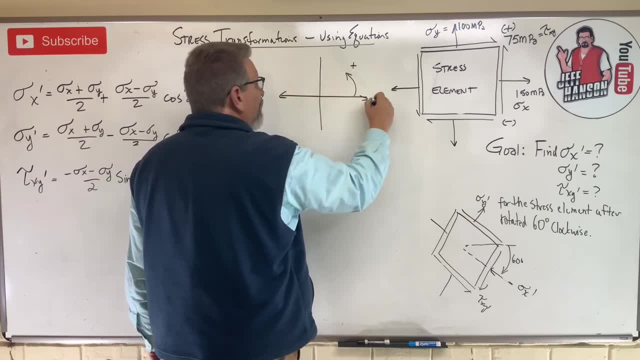 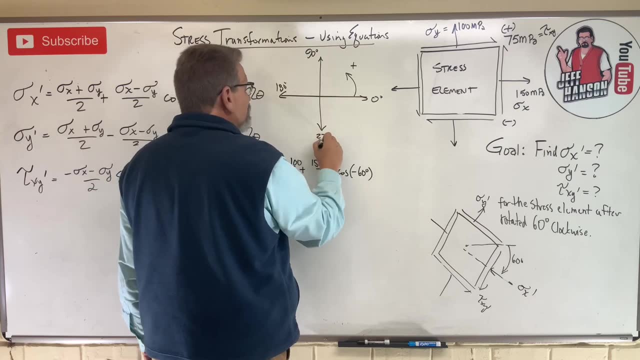 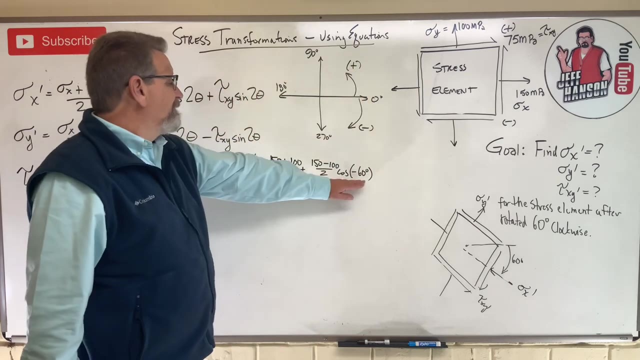 If I rotate this way, that's positive, Here's zero degrees, Here's 90 degrees. right, There's 180 to 70. So anything we rotate this way, that would be called negative. okay, So we got to put a negative 60 in there. Are you with me on that part? 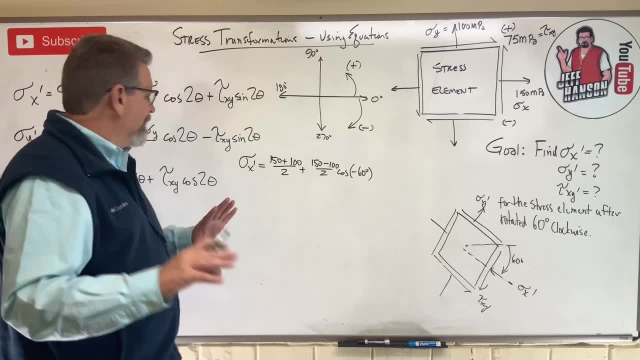 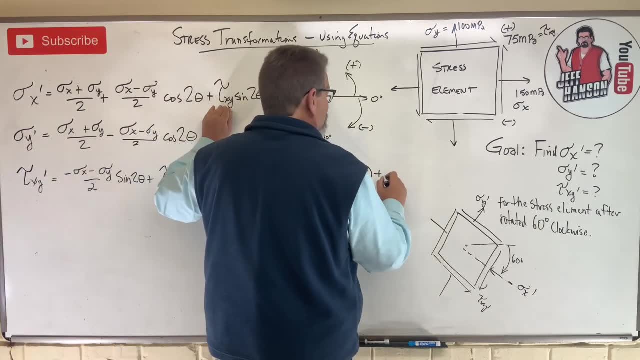 Don't mess up that. Lots of parentheses here, okay, Lots of parentheses, okay. Plus tau xy. plus tau xy is what? 75 times the sine. Oh, look what I did. I just put theta in there, didn't I? 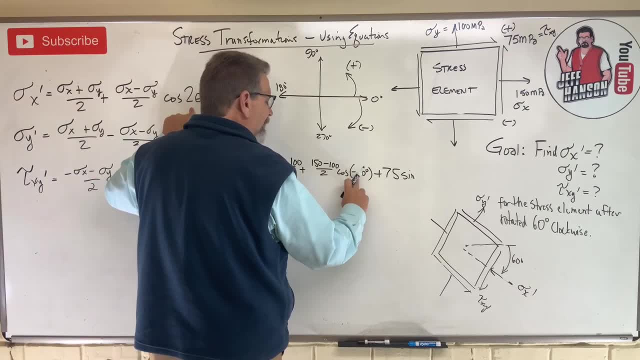 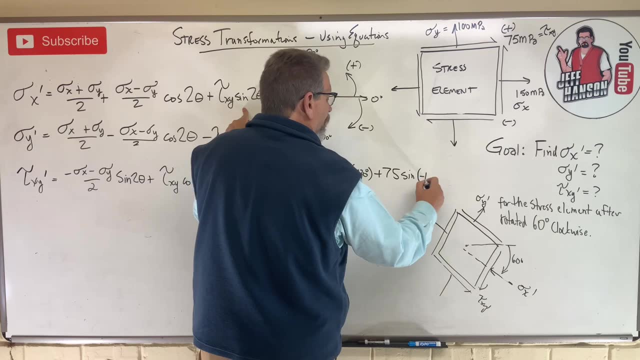 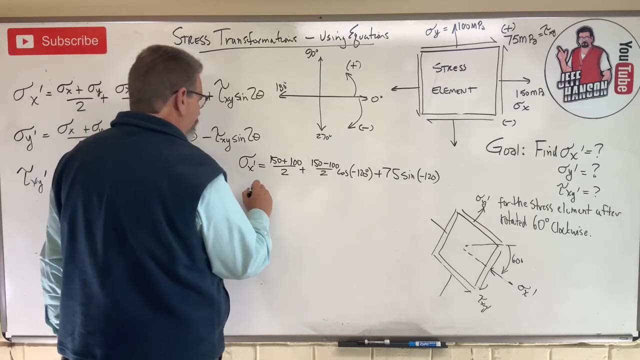 I got to put 2 theta in there. Hanson, come on man. How about 120, okay, Sine, 120, okay, Are you ready? Let's go? Here we go. So what does this equal to Sigma x prime? 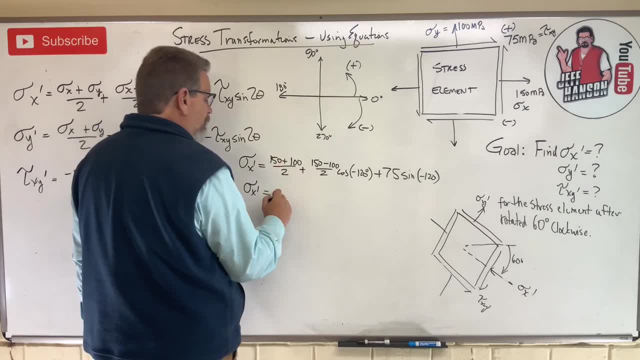 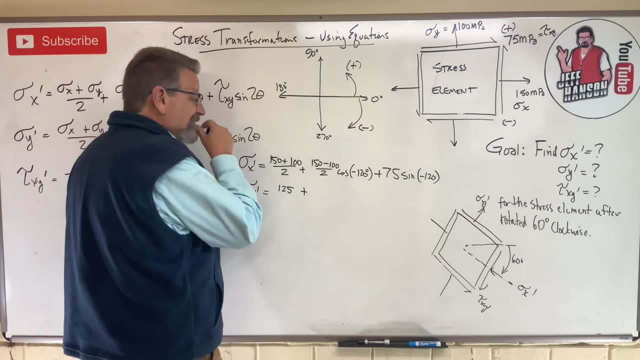 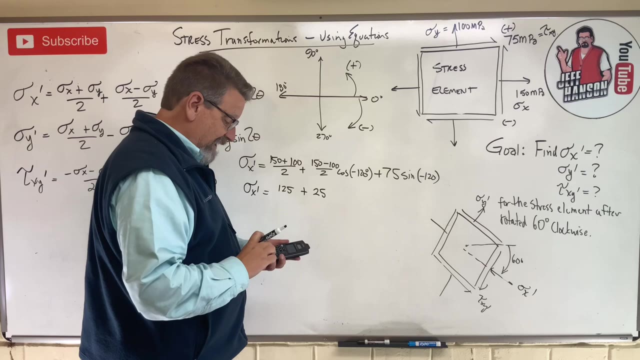 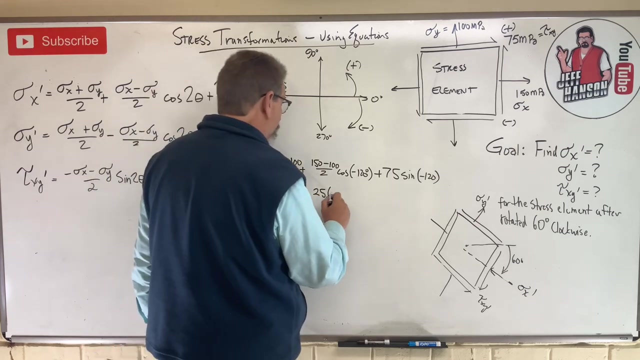 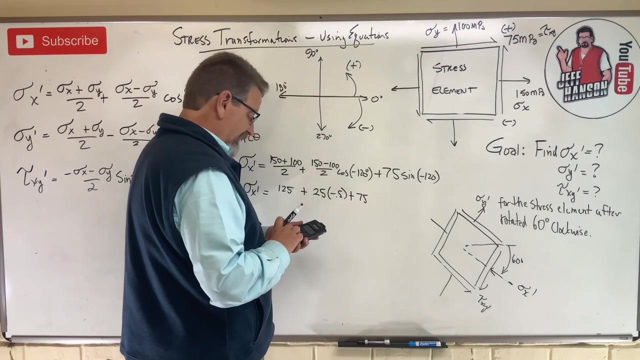 is equal to. what is that? 250 divided by 2 is 125.. And then, plus 150, minus 100 is 50, divided by 2 is 25, cosine of negative 120.. What is that? The sine of negative 120,, parentheses, oh, negative 0.5, right, Plus 75 times the sine of negative 120. 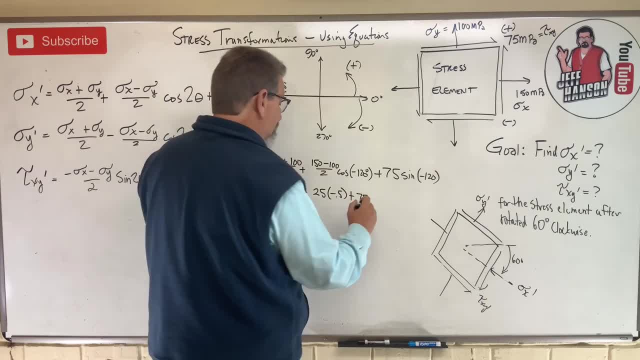 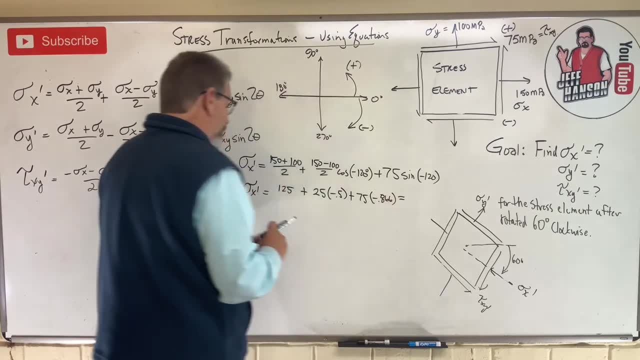 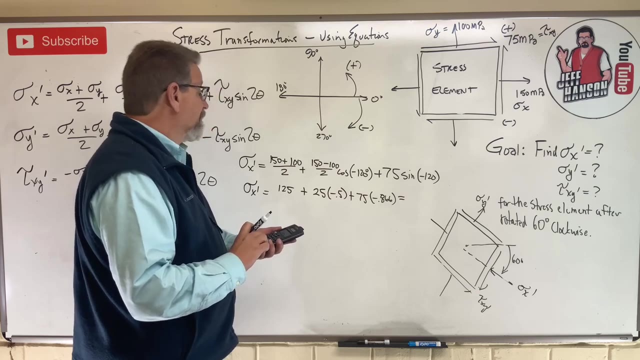 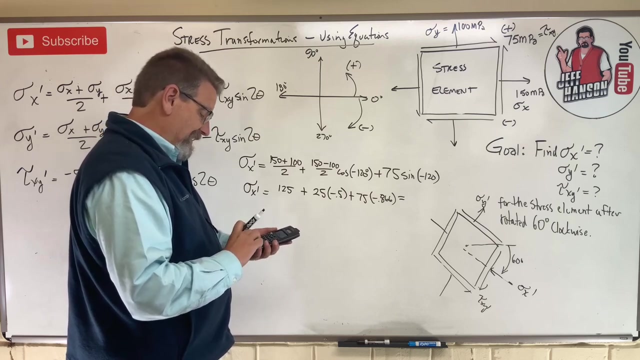 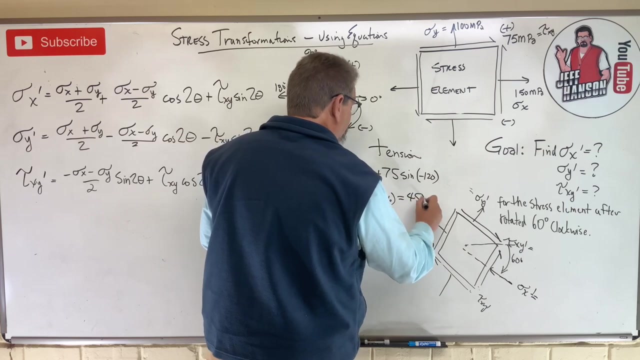 is negative 0.866,. okay. So sigma x, prime, what does that equal to? Let's add all that together Plus 25 times negative, 5 plus 75 times negative, 0.866 equals. So that's 47.55.. That's not how you write that, 47.55, and that's MPAs. okay, Be careful how you put that in there. 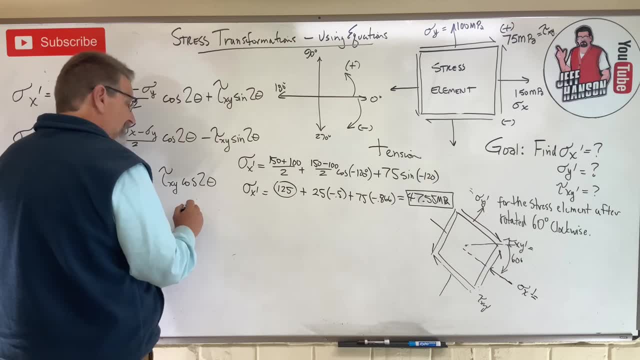 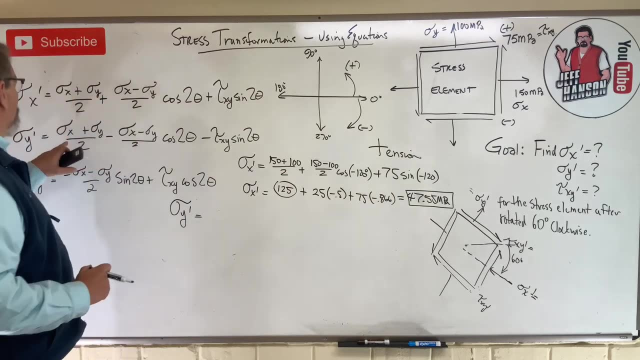 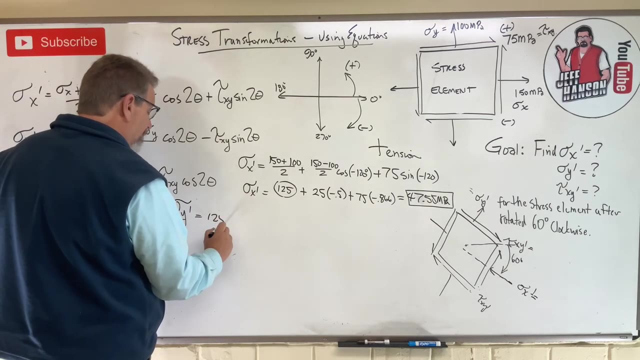 Your calculator. okay, Number, next number. next, sigma y prime. Okay, let's do this guy. What's different here? Okay, first term: sigma x plus sigma y over 2.. Hey, that's 125, isn't it 125,? 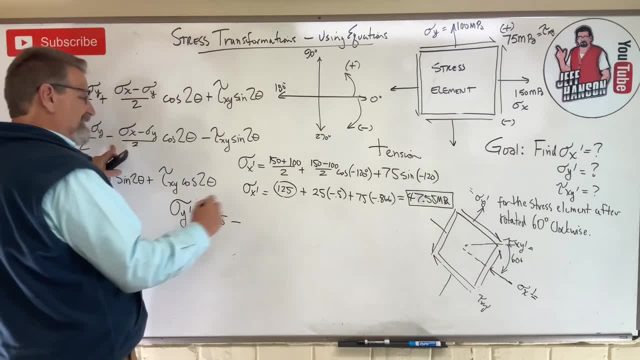 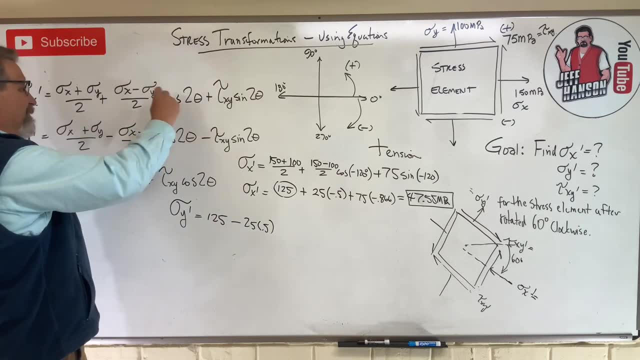 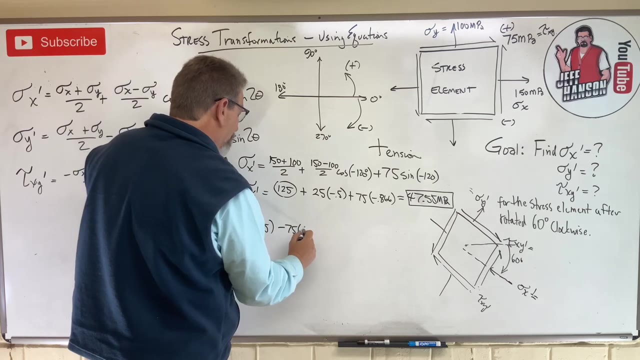 okay, Minus. everything is the same, except it's just minus, isn't it? 25 times 0.5.. Everything's the same, right? Everything Go to the next guy. Everything's the same except minus. So minus 75 times 0.866.. Okay, here we go. 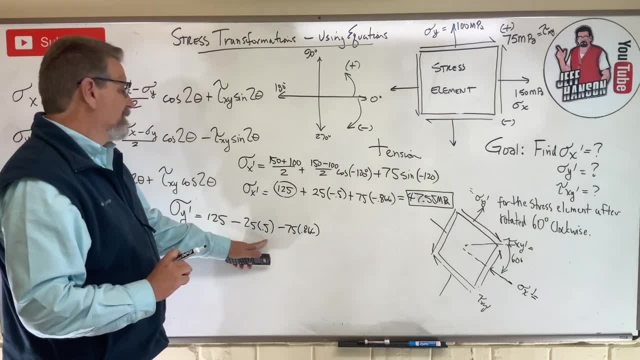 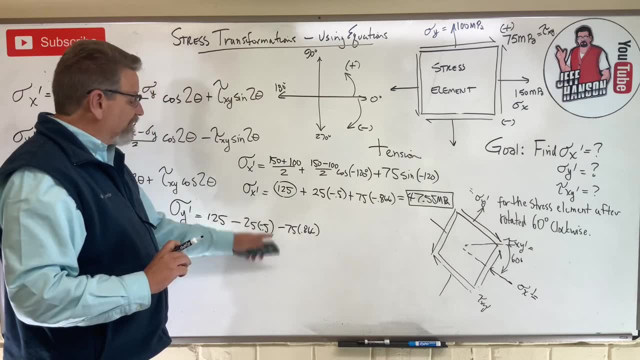 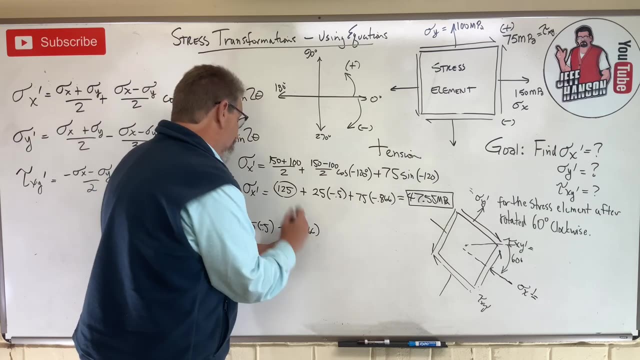 So 125 minus. oh, I forgot a minus there, didn't I? Minus and minus turns into a plus, doesn't it Plus? what's 25 times 0.5?, 12.5.. And then minus. oh, I did it again. So minus there, isn't it Minus? 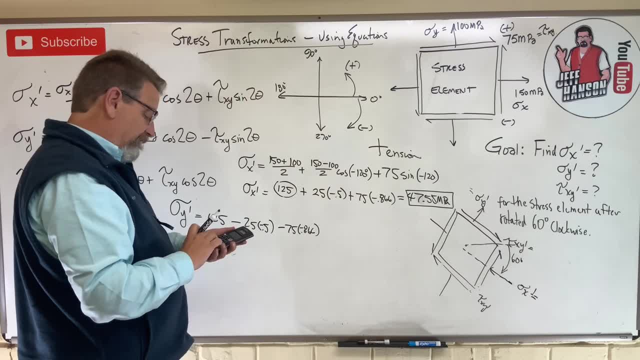 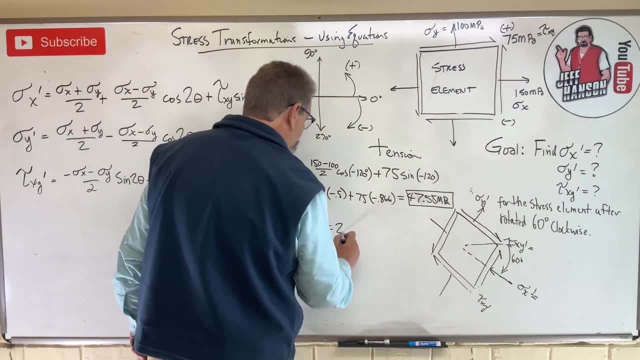 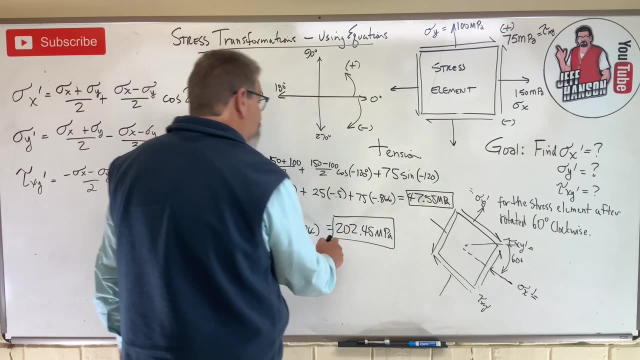 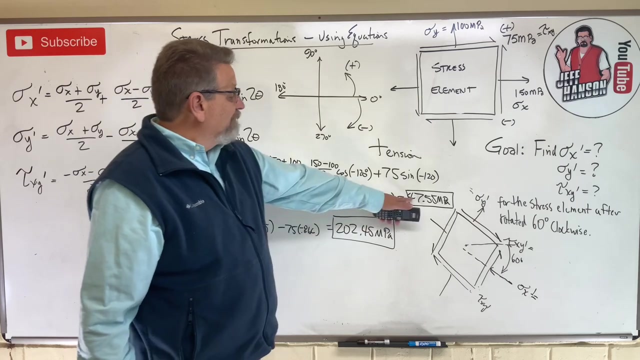 and minus. so plus again, Plus 75 times 0.866 equals 202.45 megapascals. What does the positive mean? What is positive? Remember, tension starts with a positive sign. So these being positive means that the x and the y are going to be in tension. 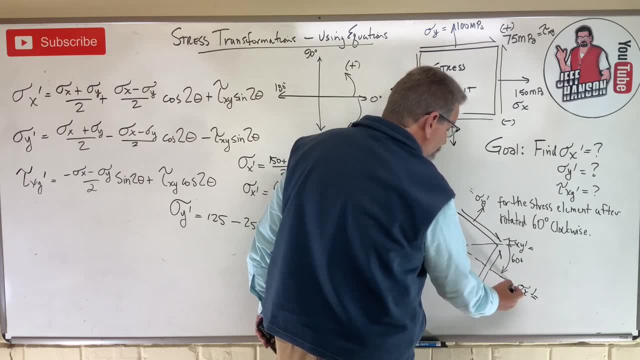 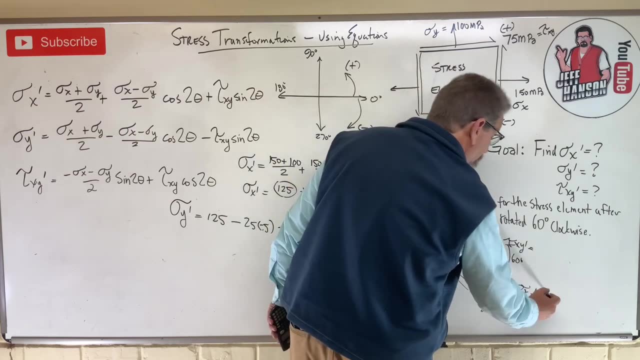 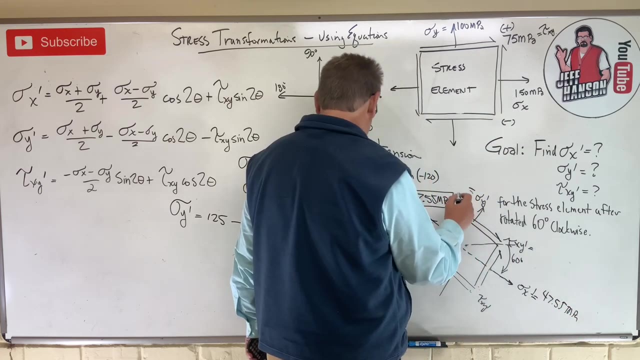 Oh, I have that one. I just guessed him a second ago, didn't I? But he's really in tension, okay, So sigma x is 47.55 megapascals And sigma y 202.45 megapascals. 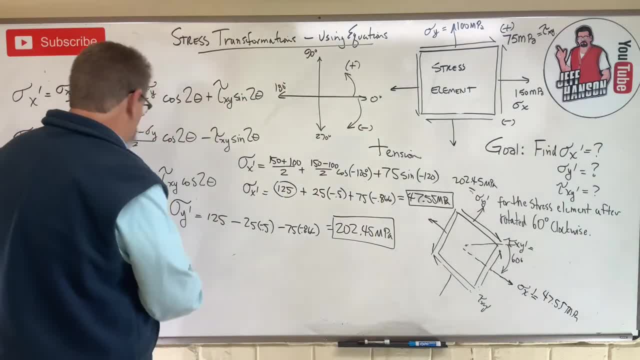 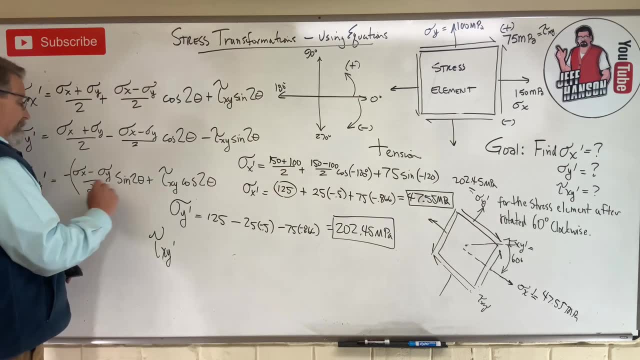 okay, Last one. let's figure tau xy prime, Tau xy prime. Now there's one tricky thing here. I should have done this to you. okay, That negative is times. it's not just times x in the numerator, It's times the whole thing there. 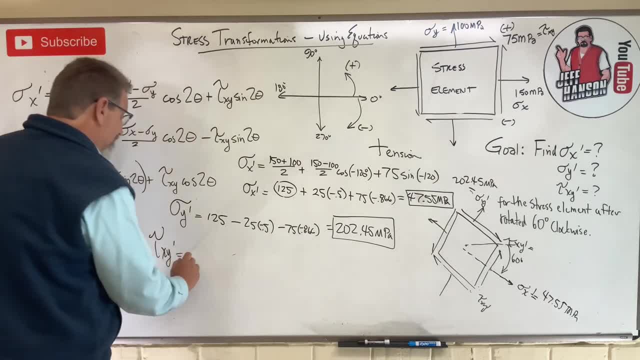 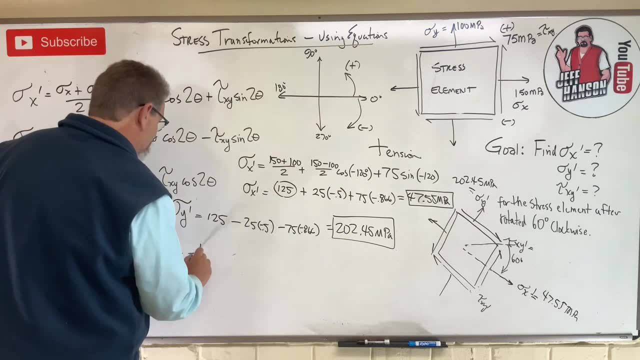 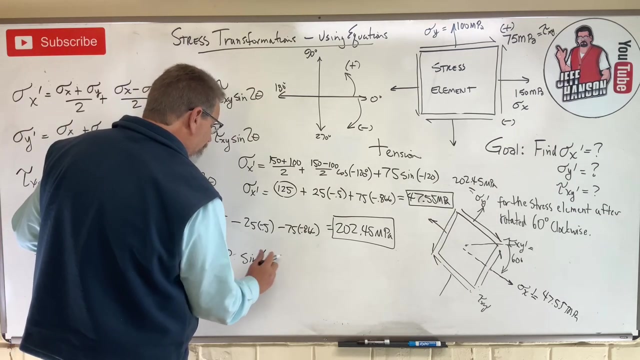 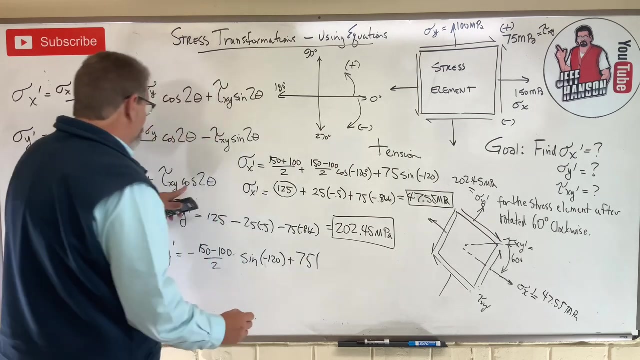 okay. So it equals negative. okay, x minus y divided by 2.. And x was what? 150 minus 100 divided by 2 times the sine of what Negative 120.. That's not how you make negatives. Negative 120,, okay, And then plus tau xy, 75 times cosine. 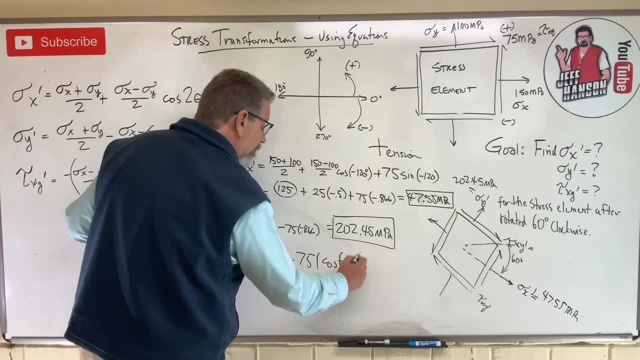 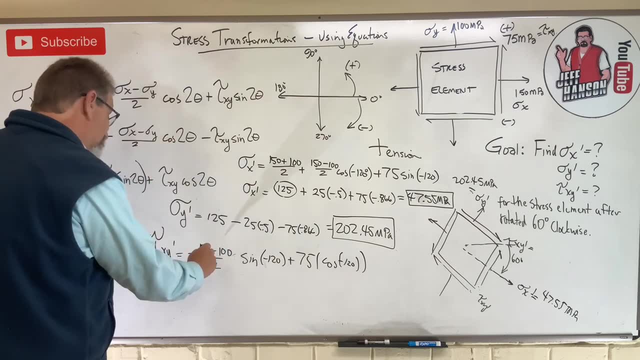 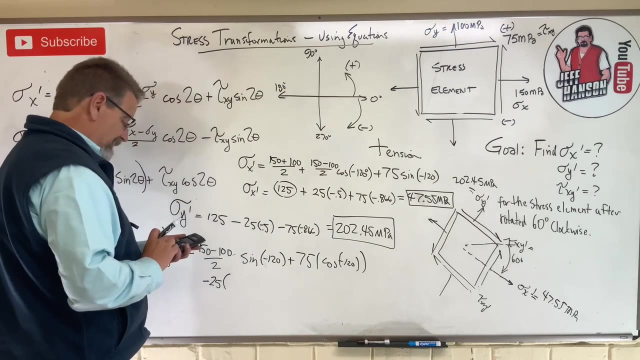 negative: 120,. okay, Let's see if we can do that. 150 minus 100 is what 50 divided by 2 is 25.. So negative 25 times the sine of. I just did this, didn't I? 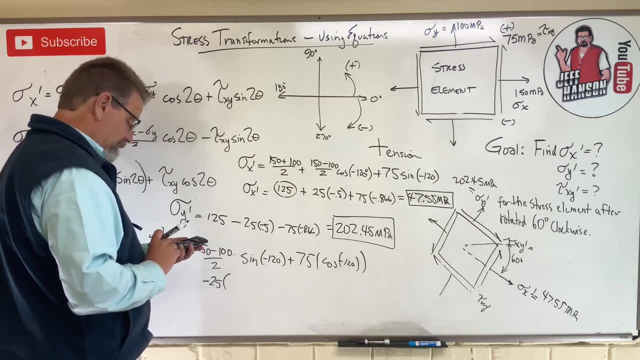 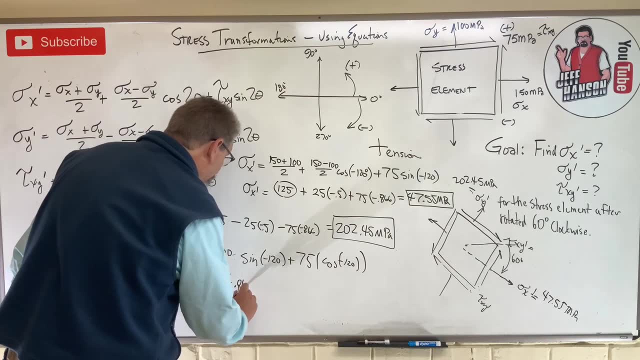 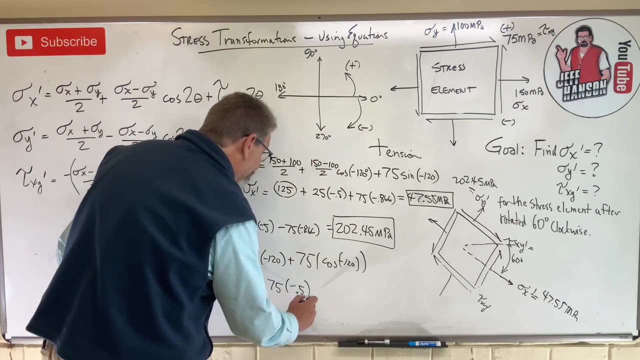 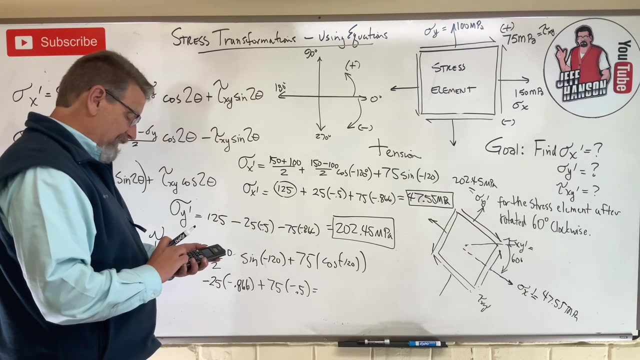 Negative 120, which is, oh no, is negative 0.866,. okay, Plus 75 times negative 0.5.. We remember that guy, at least don't we? So negative and a negative is a plus, If so, 25 times 0.866.